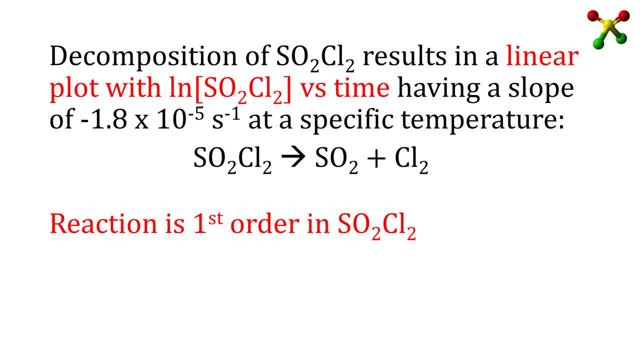 That linear plot tells us that the reaction must be first-order in SO2Cl2.. The second clue is that that linear plot has a slope of negative 1.8 times 10 to the negative 5 inverse seconds. We know that the rate constant k is equal to the absolute value of this slope. 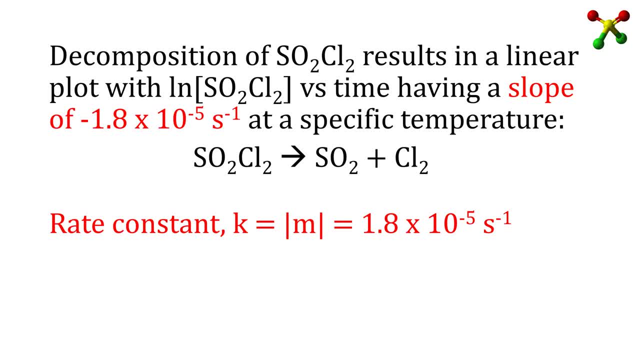 therefore, the rate constant for this reaction is 1.8 times 10 to the negative 5 inverse seconds. Our third and final clue is that the units of k and the units of slope indicate that this reaction is first-order in SO2Cl2, since the units are inverse seconds. 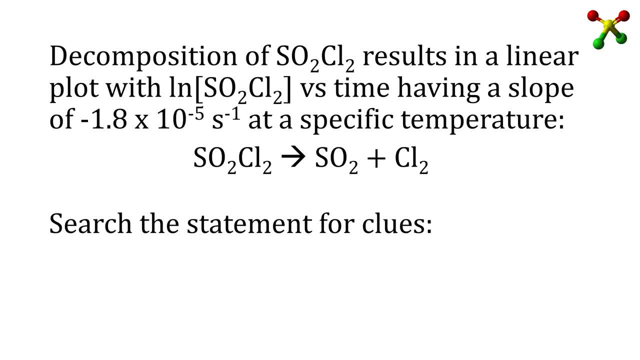 So, in summary, before we solve any problems, we first search the statement for clues. we find the reaction is first-order in SO2Cl2 and we find the rate constant is 1.8 times 10 to the negative 5 inverse seconds, is 1.8 times 10 to the negative 5 inverse seconds. The first problem we'll 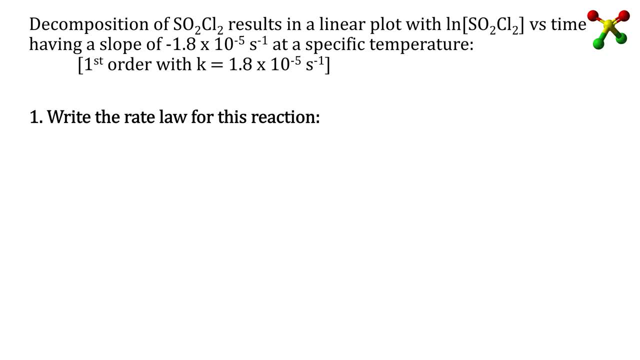 solve here is to write the rate law for this reaction, Since the reaction is first-order in SO2Cl2, and that's the only reactant. the rate law then is: rate equals K times the concentration of SO2Cl2 to the first power, or simply K. 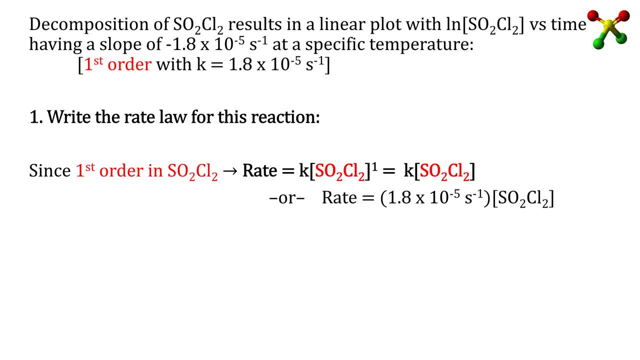 times SO2Cl2.. You may also see a rate law written with K, the rate constant numeric. In that case it would be: rate equals 1.8 times 10 to the negative 5 inverse seconds times SO2Cl2 concentration. The next problem is to 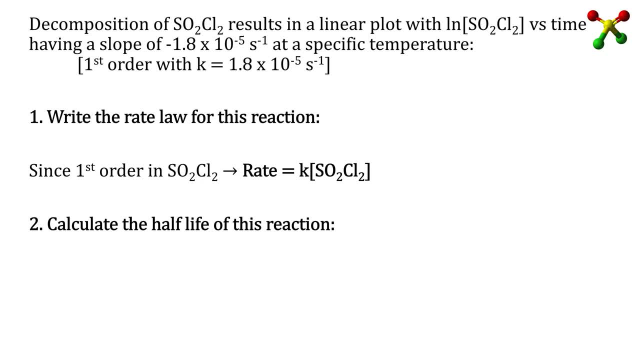 calculate the half-life for this reaction. Since this is a first-order reaction, our half-life is simply 0.8 times 10 to the negative 5 inverse seconds. Notice that the half-life of this first-order reaction is independent of initial concentration of reactant. In contrast, 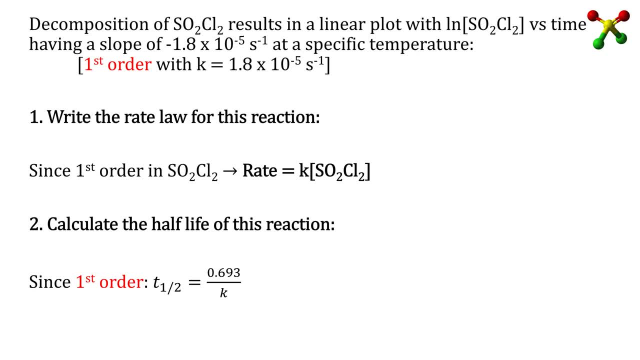 the zero-order and second-order half-lives are dependent on initial concentration. We plug in our rate constant and we find that our half-life is 38,500 seconds or, correctly rounded to two significant digits, 39,000 seconds. The third problem asks how long will it take for SO2Cl2 to decrease to 25% of its? 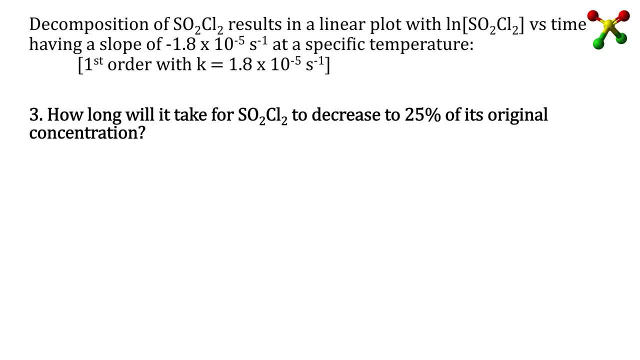 original concentration. The key step needed to solve this problem is to recognize that the SO2Cl2 concentration at time t, which we don't know yet, is equal to twenty-five percent or 0.25 times CO2, storms times CO2-divided by the. 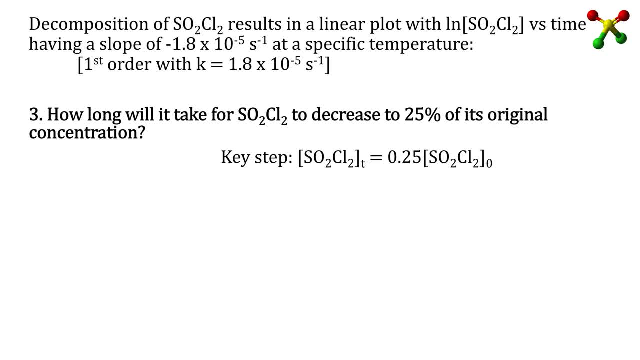 the initial concentration of SO2Cl2.. We'll use the integrated rate law for a first-order reaction, as shown here and simplified with A representing SO2Cl2.. We need to rearrange this equation to solve for T. To do that, we'll first put 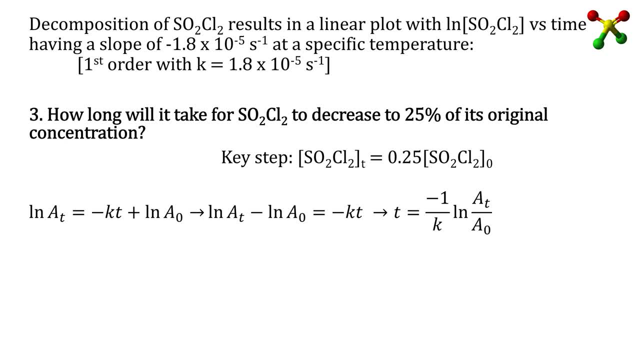 both natural log terms on the same side and then we'll recognize that T is equal to negative 1 over K times the natural log of our reactant concentration at time. T divided by our initial reactant concentration, That means for this problem, T is equal to negative 1 over K times the natural log of SO2Cl2 at time. 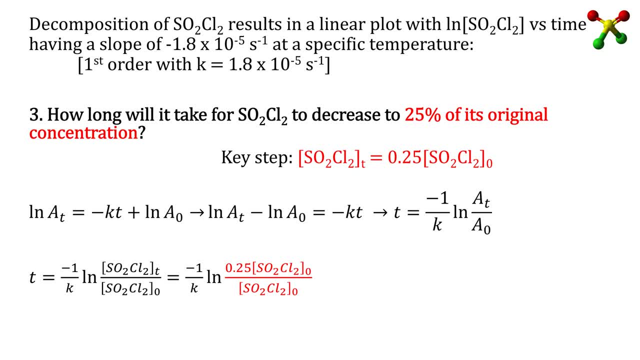 T divided by the concentration of SO2Cl2 initially. Using that key step shown above, we can reduce this to time equals negative 1 over K times natural log of 0.25 SO2Cl2 initial divided by SO2Cl2 initial. 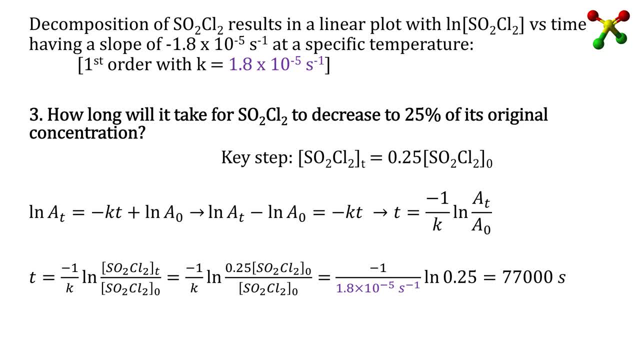 Those initial concentrations of SO2Cl2 will cancel and we'll plug in our rate constant and we'll find that negative 1 divided by the rate constant times the natural log of 0.25 gives us a total of 77,000 seconds. 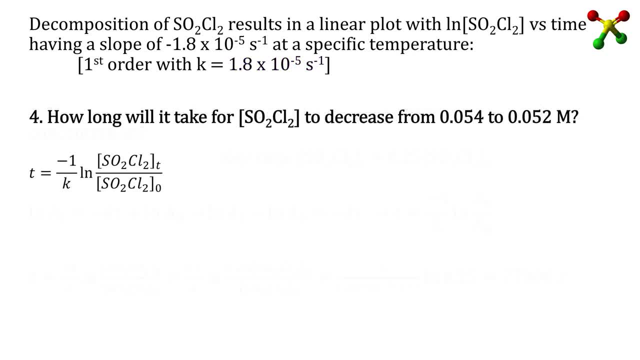 The fourth problem we'll solve is to determine how long it will take for the SO2Cl2 concentration to decrease from 0.054 to 0.052 molarity. We'll use the first-order integrated rate law, again solved for T, as we did in the previous. 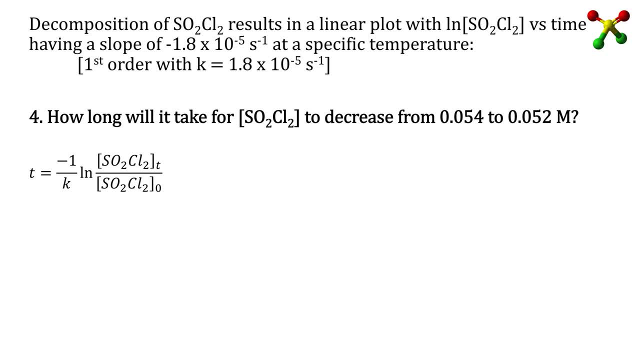 problem and we'll plug in the concentrations for SO2Cl2 both at time T and at time 0, initial. When we do that and include our rate constant, we find that our time for the SO2Cl2 to decrease to 0.052 molarity is 2,100 seconds. again, correctly rounded. 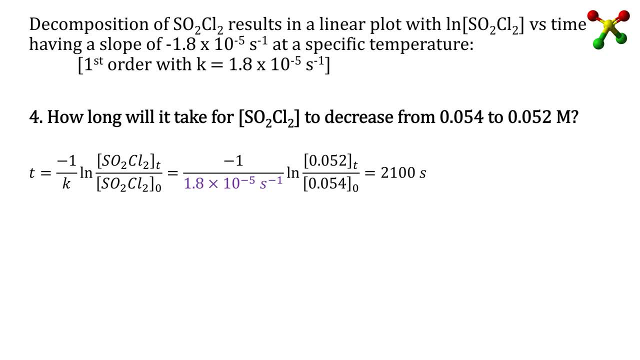 to two significant digits. The next problem states: if SO2Cl2 concentration starts at 0.0105 molarity, we'll have the concentration at 0.02, so for the second algorithm, КdC2, byuso superimposed. 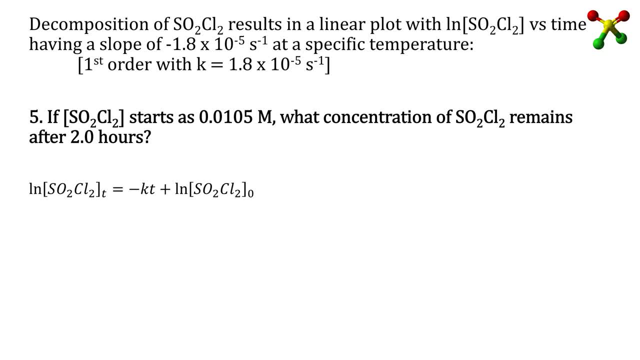 definitely missed our four instances. LaBET, têm, Lb. You can see the amount of concentration. what concentration of SO2Cl2 remains after 2.0 hours? We again return to the integrated rate law equation for a first-order reaction And we insert our rate, constant and our time and our initial SO2Cl2 concentration. 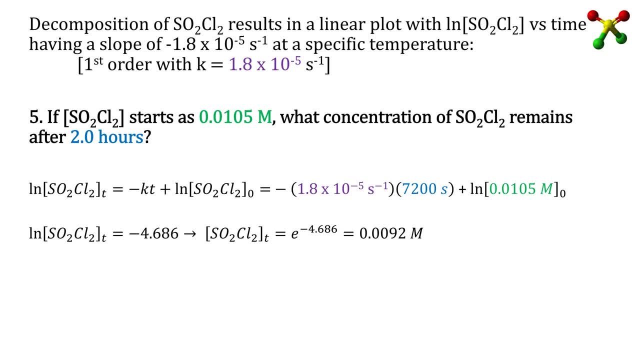 When we do this, we find that the natural log of our SO2Cl2 concentration at time t, which is 2 hours, is equal to negative 4.686.. That's not my final concentration. In order to do that, I need to remove the natural log. 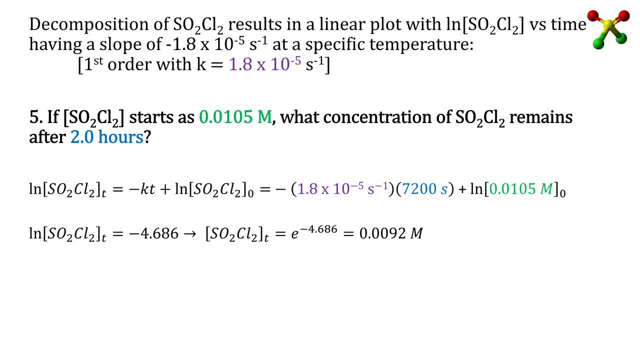 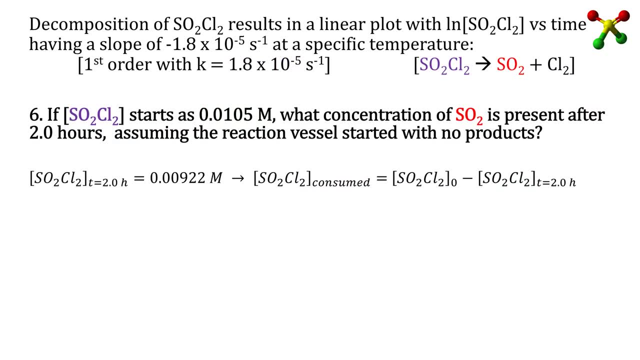 and I find that my SO2Cl2 concentration after 2 hours is 0.0092 molarity. Our sixth and final problem is: if SO2Cl2 concentration starts at 0.0105 molarity, what concentration of SO2 is present after 2 hours? 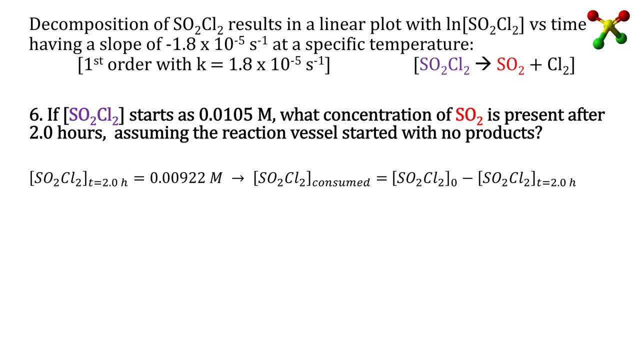 assuming the reaction vessel started with no products, We recognize that our SO2Cl2 concentration at time equals 2 hours is equal to 0.00922 molarity, as calculated in the previous step. I've added one digit beyond the 0.00922 molarity.